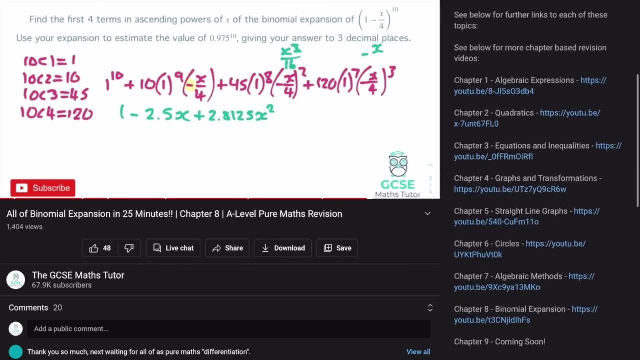 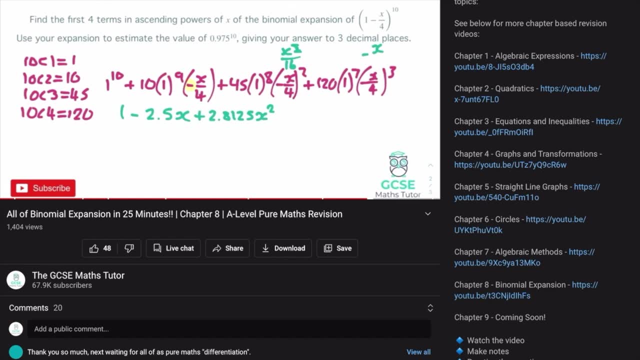 I cover all of the ASPure curriculum and if you scroll down you can also see all of the chapters. Now these will slowly be filling up until it has filled the entire ASPure curriculum. so hopefully by the time that you are watching this video, all of them will be actually in the 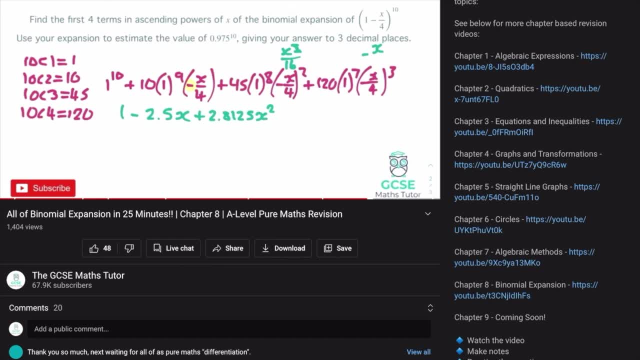 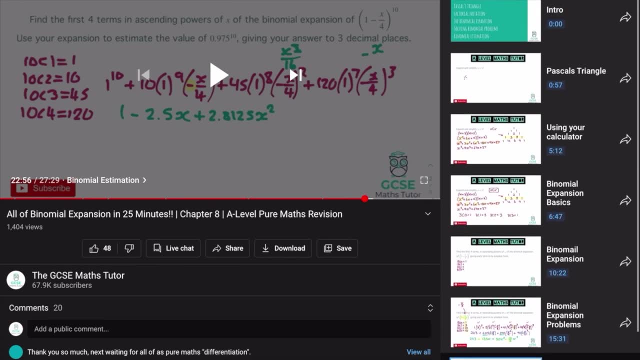 description and you can click and watch each chapter. If you click onto the video and click the link in the bottom left, there you can actually see all of the chapters that are within this video as well, So you can skip through and have a look at the pieces of that chapter that. 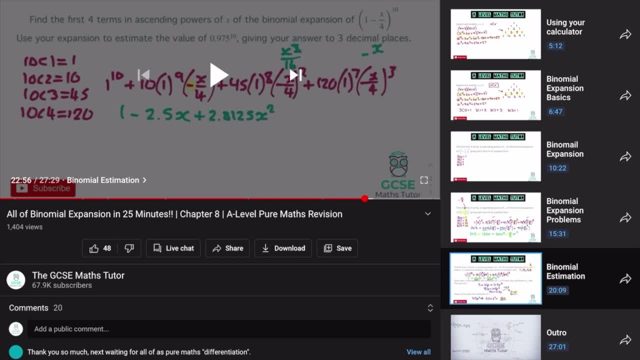 you are needing to have a look at for your revision. So that's how this video works. hopefully that's useful and helpful. If you enjoy this video, please don't forget to like the video. don't forget to share it with some of your friends. but with that being said, let's get started. 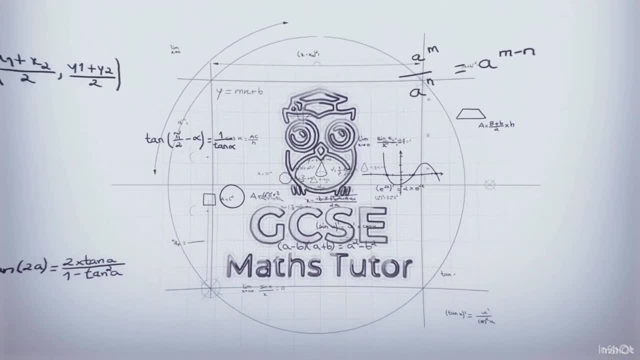 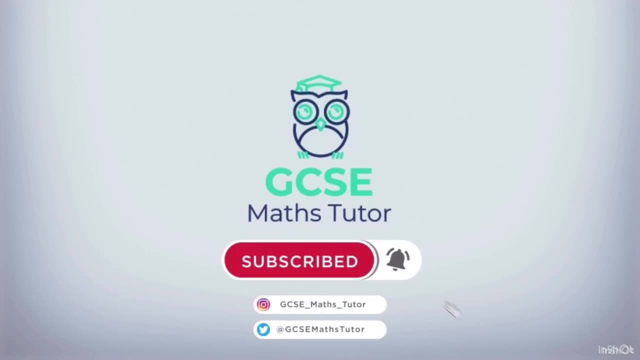 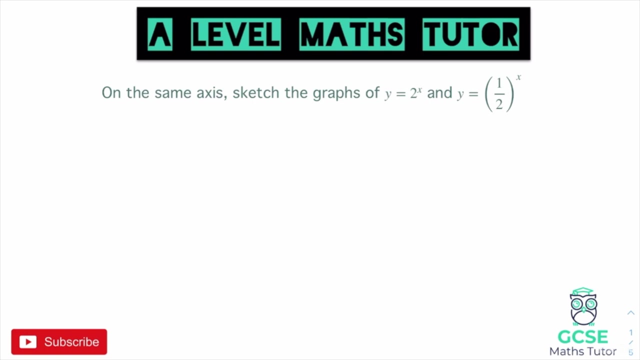 Okay. so when having a look at exponential graphs, it's important that we're able to sketch them. So this question says: on the same axes, sketch the graphs of y equals 2 to the power of x and y equals a half to the power of x. So if we draw a little sketch of some axes we can think about, 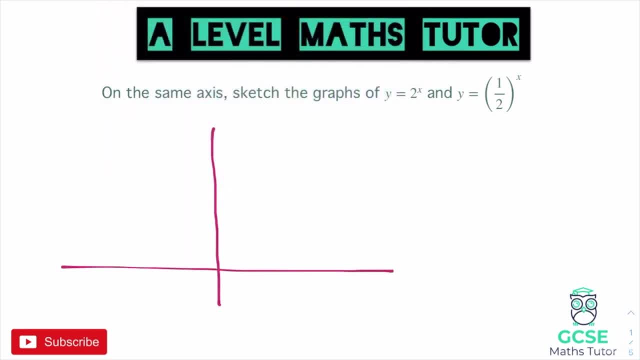 what these would look like. Now for the first one we will sketch. y equals 2 to the power of x. Now, this is an increasing function here, so it would be sloping upwards, and again with an exponential function, the graph approaches but never touches zero. So this would be our: y equals 2 to the power of x. and now we'll. 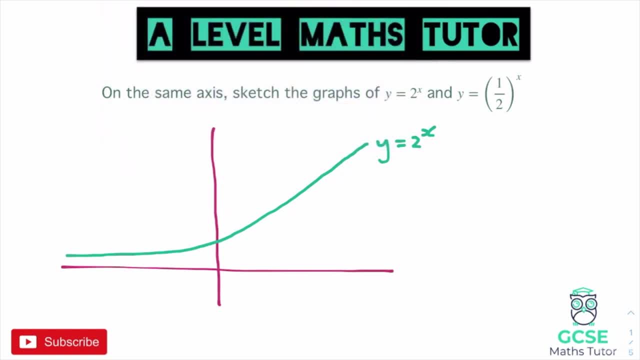 have a look at: y equals a half to the power of x. So for y equals a half to the power of x. that is a decreasing function, So it would be sloping downwards. Now it would look very similar to this, but it would just be sloping the other way and, as you can see, it is decreasing and again getting. 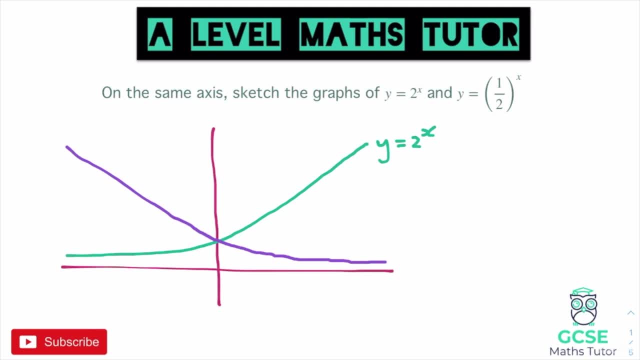 closer and closer to it, approaches, but never touches zero. So this one here would be: y equals one half to the power of x- There we go, put that in a bracket- and to the power of x. Now, as with all exponential functions, there are a couple of things that you need to be aware of. So for these, 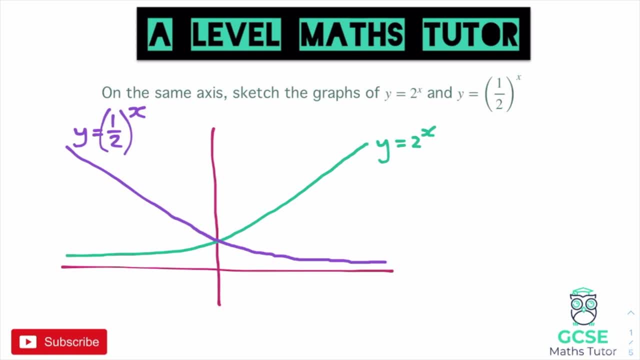 exponentials here. if we were to put in an x value of zero, which is what's on the y axis, there we a y coordinate just here of one. Anything to the power of zero is one, so that's something to be aware of. Another thing that we should be aware of as well is that we have an asymptote Now. this 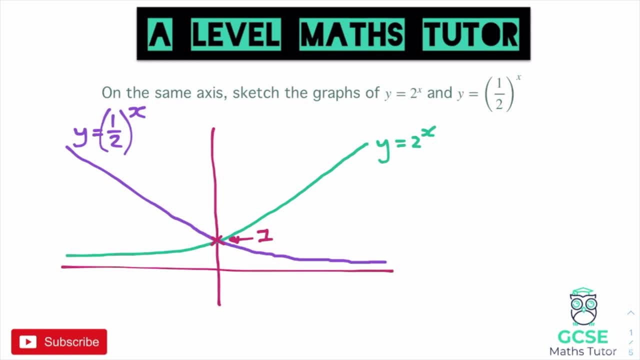 here never actually touches the x axis. so the x axis is our asymptote. Now for this one. here the equation of the x axis is: y equals zero. So our asymptote of these graphs- and we'll just label that there- Asymptote. there we go. 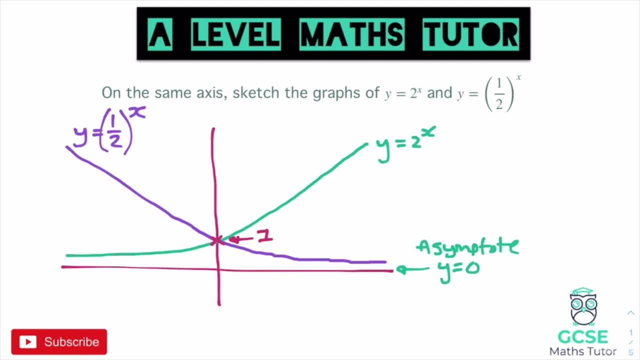 Asymptote is: y is equal to zero. Of course that would change if we put a graph transformation in something like two to the power of x plus five would move the graph upwards by five, which would move our y intercept and would also change our asymptote. But there we go. that is looking at. 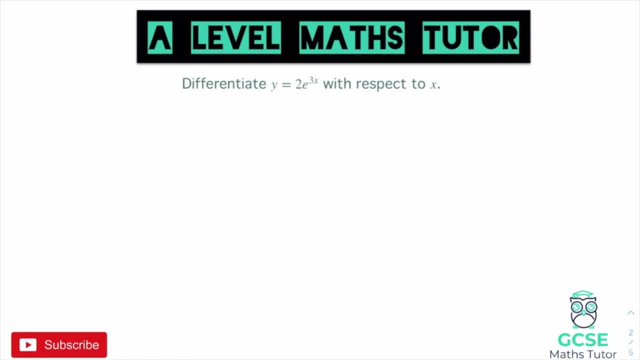 sketching exponential graphs. So when it comes to differentiating an exponential, there is just a few rules that we need to know. So this question here says: to differentiate y equals two e to the power of three, x with respect to x. Now, if we are going to differentiate this, 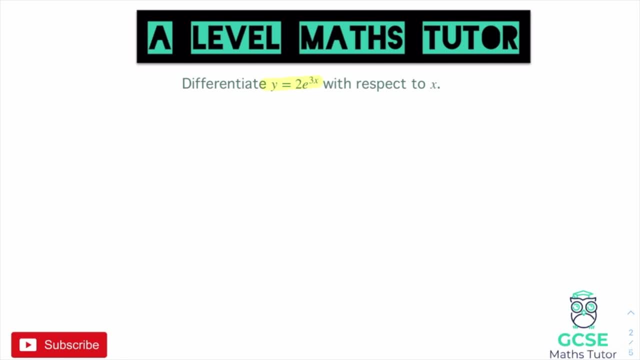 all we actually have to do is do it in a similar way to how we differentiate, but just one little thing changes. So when we do the differential, so dy over dx- of this exponential, we multiply the coefficient of e by the coefficient of the x. So that means we are just going to multiply the two. 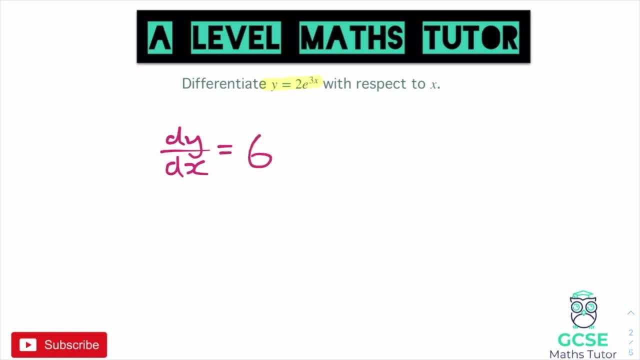 by the three. So if we do the differential this time, which makes it six, we still have e and the power stays the same. So that is just still going to be a power of three x. So if at any point, you have to differentiate an exponential, this is all that you need to do: Multiply the coefficient of e by the. 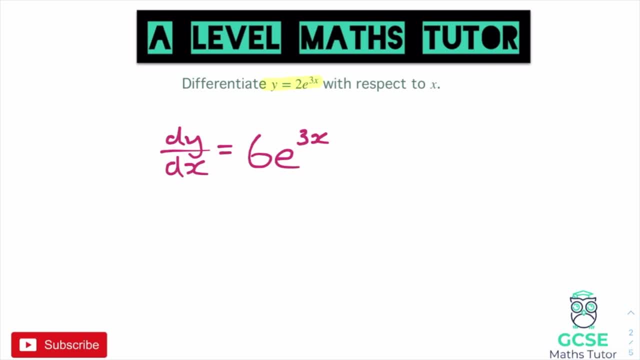 coefficient of the x in the power and then keep the power the same. So differentiating an exponential is quite nice and simple. Okay, so when we are solving an equation with an exponential- and we are at this question here- says to solve the equation e to the power of two x plus three. 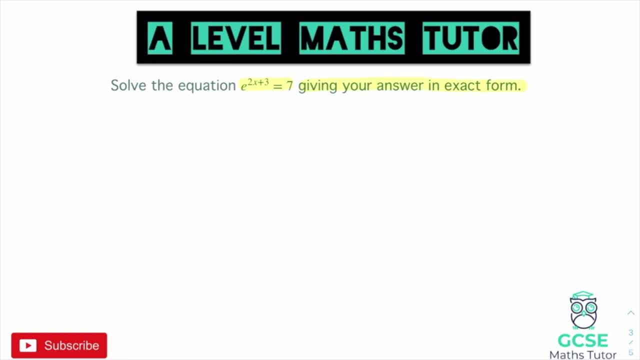 is equal to seven and we are going to give our answer in exact form. And this is when we start to use natural logarithms. So in order to remove the e at the start, we take the natural logarithm of both sides. Now the natural logarithm is just the inverse of our exponential there. So if we 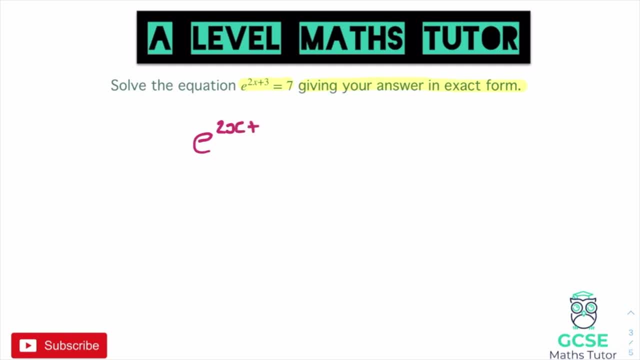 write this out: e to the power of two x plus three is equal to seven. We take our natural log of both sides. the e disappears, we get two x plus three and that is going to be equal to the natural log of seven. So it's quite nice and easy to get rid of the. 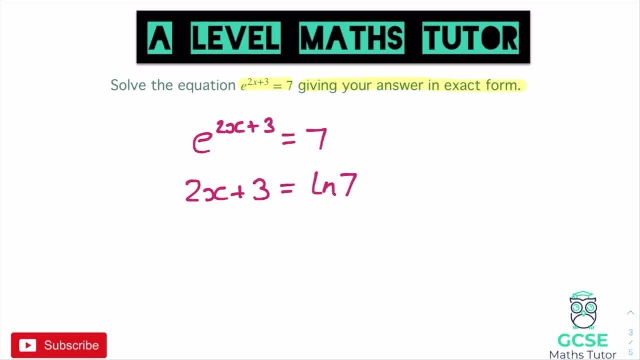 exponential. All you need to do is take the natural log of both sides and essentially it just drops the power down. Now we can just solve it like a normal equation. So we would take away three from both sides, which would leave us with two. x is equal to the natural log of seven. take: 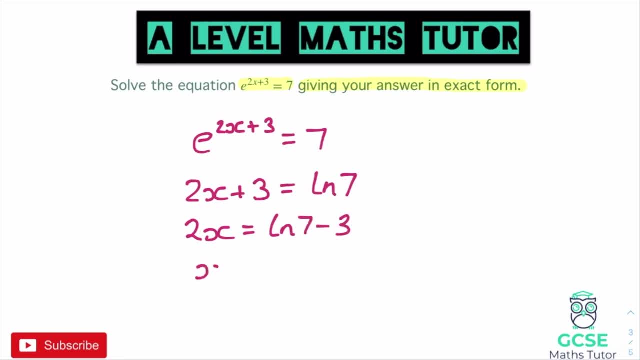 away three, And then we would divide both sides by two. So x is equal to the natural log of seven minus three, all divided by two. Of course that could be written in a different way. We could put that divided by two in front of both, So we could say a half of log seven minus a half of three, which 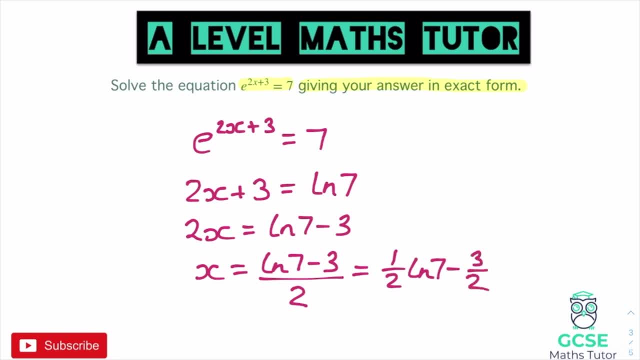 could just be written as three over two, So either one of those would be fine as our answer. I tend to write my answer like this most of the time, So I do prefer that one on the right, But both of those answers there are fine and we have given our answer in exact form as we have. 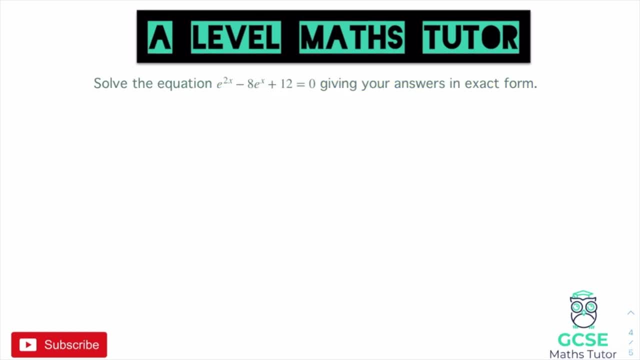 left the natural log within our answer. Okay, so another type of equation where we're going to be using natural logs. So for this particular one here you can see what we actually have is an exponential quadratic here, and we're just going to have a look at factorizing it in order to find 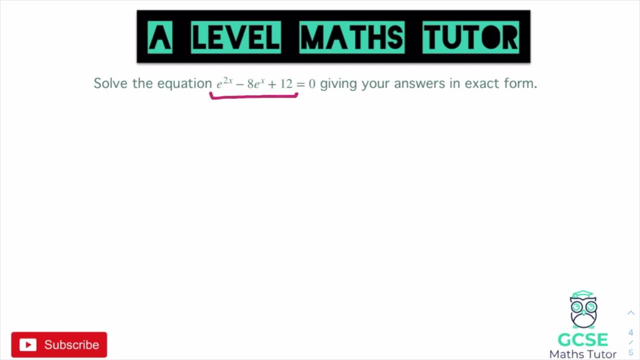 our solutions. So it says: solve that equation: e to the power of two x minus, e to the power of x plus twelve to the power of two x minus, e to the power of x minus twelve. So we're going to have: a is equal to zero and again giving your answers in exact form. So for this question here it does. 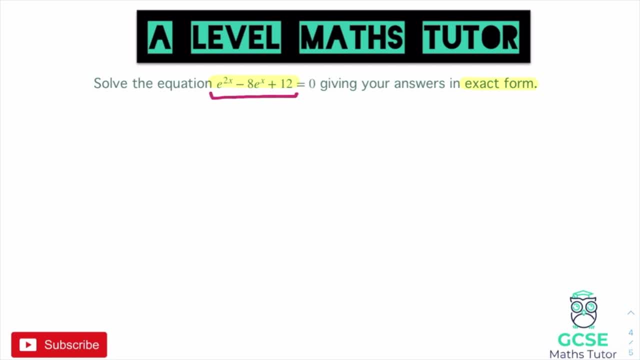 give us a bit of a hint that we're going to be using natural logs and to start with we just need to factorise it. So at the start of both of our brackets we will have e to the power of x, as when you expand that e to the power of x multiplied by e to the power of x would equal e to the power of. 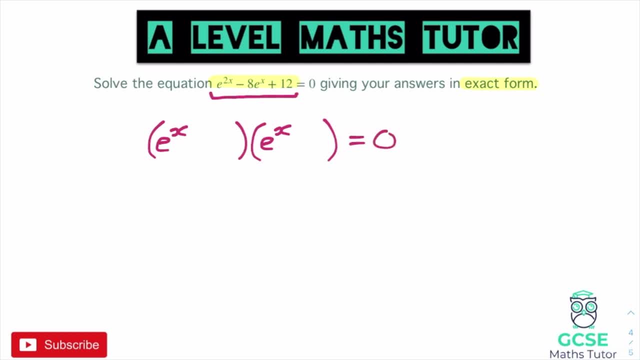 2x, and that is all equal to zero. Of course, if it wasn't equal to zero, you may just have to rearrange these first. but once we've got it into that form, we can now factorise. So looking at the 12 there: 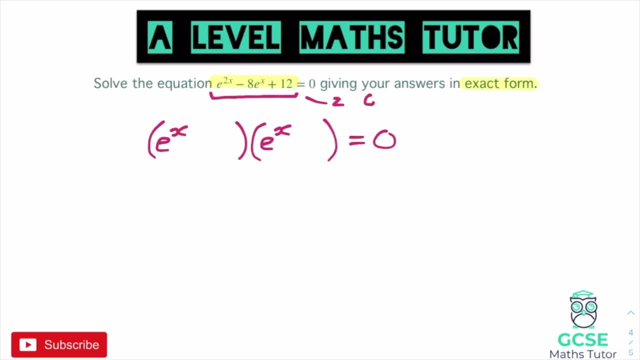 we could have some factors. we're trying to make 8 in the middle, so 2 and 6 is going to work. So in our bracket we'll have minus 2 and minus 6 and that would equate to negative 8. e to the power of x in. 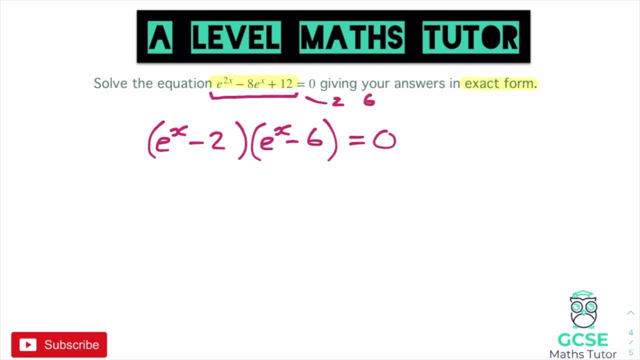 the centre there. So we have two solutions. for the first one we have e to the power of x has to be equal to positive 2, and here we have e to the power of x has to be equal to positive 6.. Now, before we just go ahead and solve that just as a side note, when we have this here: e to the power. 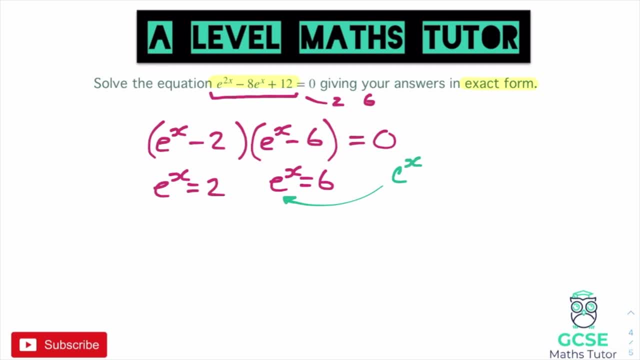 of x has to be positive. Okay, e to the power of x must be positive. and that means if we do get an answer which says e to the power of x is equal to negative 3, for example, we would have to discard that answer and we would just use the 1.. But this one here we have, both being positive e to the power. 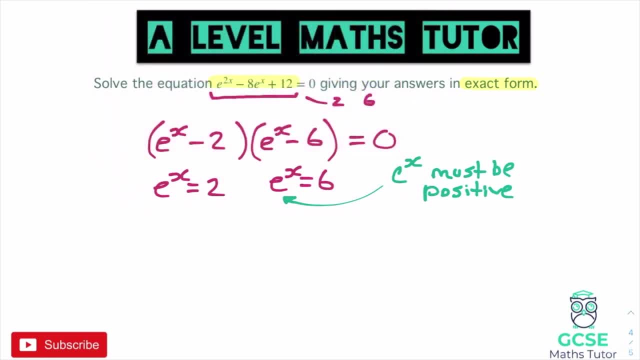 of x equals 2, and e to the power of x equals negative 3.. So we have e to the power of x equals 6.. So these are both going to be solutions, and it does give you a little bit of a hint here, as it. 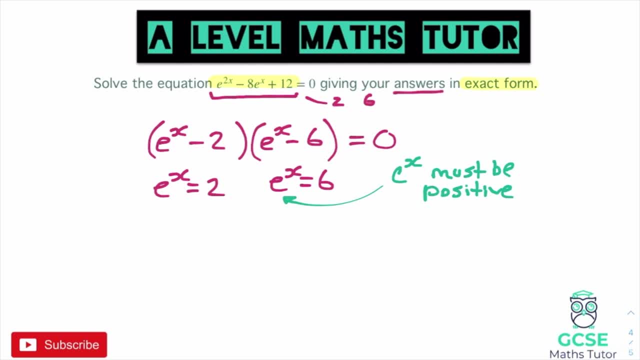 says the words answers. So for this one we now just take the natural log of both sides. So for the first one on the left there, x would equal the natural log of 2 and x would equal the natural log of 6, and again they are both in exact form. so we would leave our answers like that. So e, x equals. 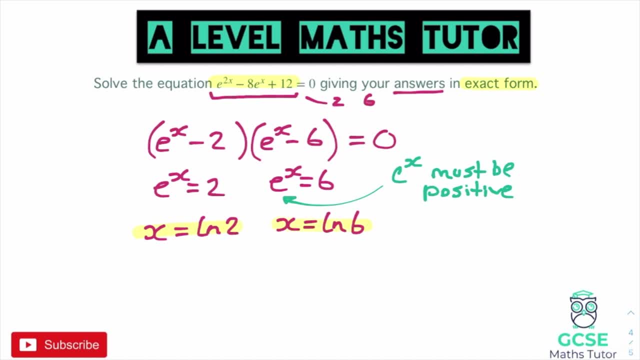 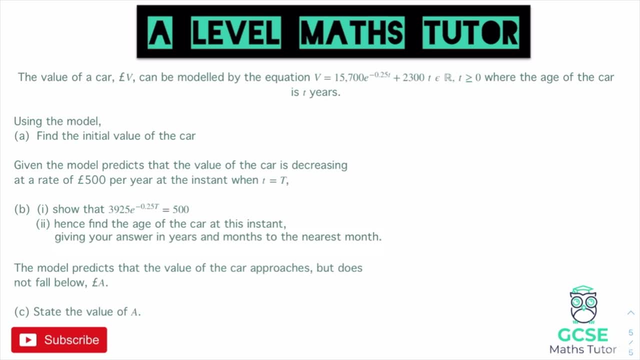 the natural log of 2 and the natural log of 6.. Okay, so when we are having a look at modelling with exponentials, the questions do get quite tricky. So it says here: the value of a car, and that is in v pounds, can be modelled by the equation. 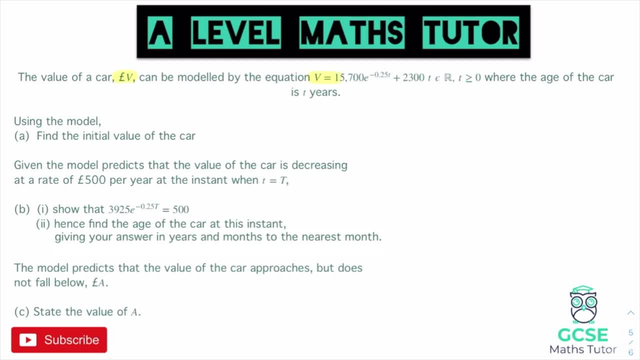 v is equal to 15,700, e to the power of minus 0.25 t plus 2,300, where t is a real number and t is greater than or equal to 0, where the age of the car is given to us in t, So we have a real number. 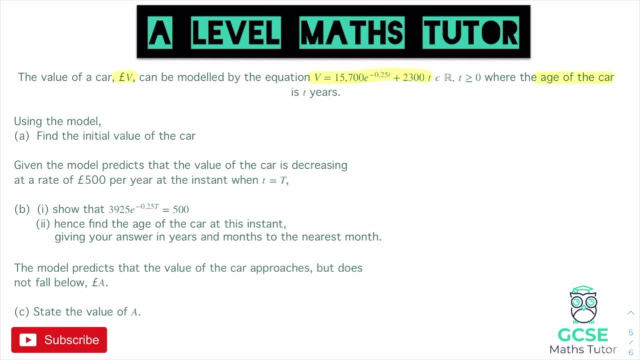 of t years. Always worth highlighting that the age of the car is t years, just so we don't forget about that. So it says here: using the model, find the initial value of the car. Now, the initial value of the car would be found when t is equal to 0. So all we need to do to find the initial value of 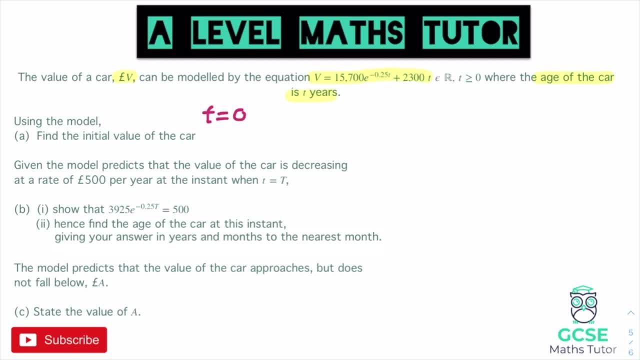 the car is. substitute t equals 0. into our equation and see what we get. Now, if we do substitute t equals 0, we would have 15,700.. e to the power of a negative 0.25 t times 0 is just going to equal 0.. Now anything to the power. 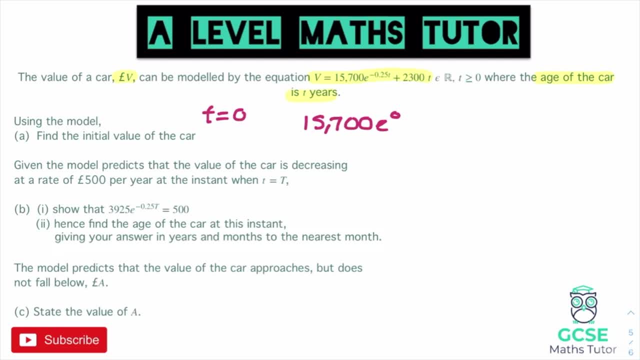 of 0 is 1, so that is just going to be 15,700.. We then have to add 2,300 to that and that means we just have 15,700 plus the 2,300, which gives us a final answer of- and it's in pounds. so we would say: 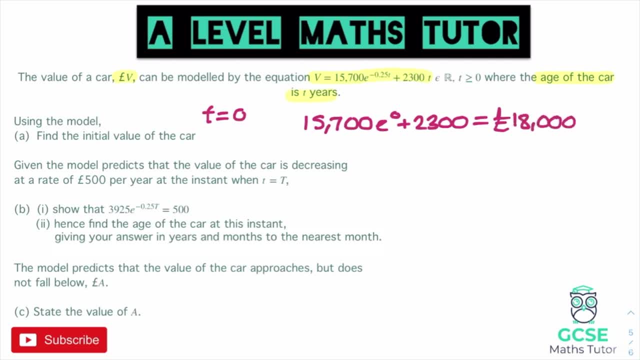 18,000 pounds And that would be the initial value of the car. So we'll just underline that as that's our first answer. On to part b, it says: given the model predicts that the value of the car is decreasing at a rate of 500 pounds per year, at the instant where the time is equal to capital, t show that. 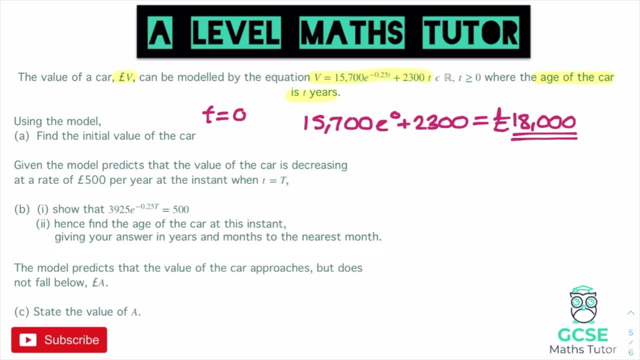 3,000, and let's just highlight this: 3,925 e to the power of negative 0.25 capital t is equal to 500.. So, in order to look at this, we would want to differentiate that as we are looking at the rate. 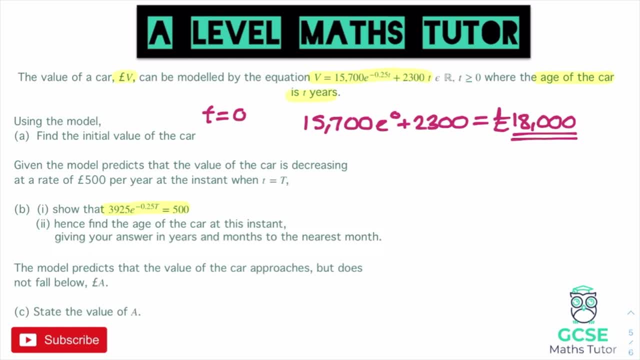 of change, or the gradient there, when it is going down by 500.. Now, also just taking note here, if it is going down by 500 pounds per year, that would be a negative 500 as our gradient. So in order to find this, we're just going to want to differentiate it to start with. So we're going to differentiate. 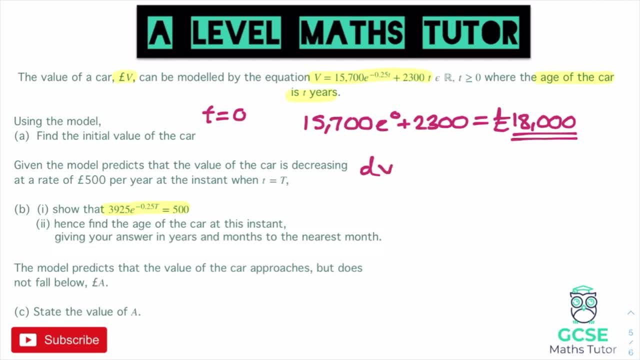 v and we're going to do that with respect to t. So if we differentiate d, we have v by dt, and we are going to be doing this at the instant where t is equal to capital T. So we're just going to replace the little t with big T in our differential. So if we 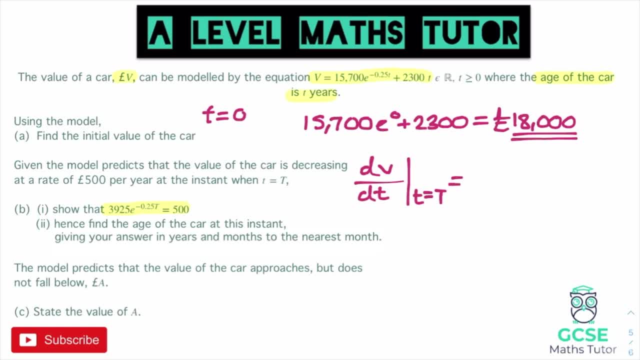 go about doing that here. let's have a look at what we get. So we're going to multiply 15,700 by negative 0.25. And if we type that into our calculator, we get negative 3,925 e to the power of negative 0.25.. Now if we do this again, we get negative 3,925 e to the 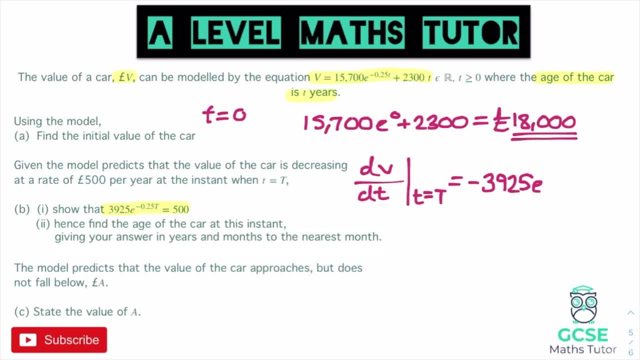 the power of- and don't forget when you're differentiating an exponential. the power is not going to change, so it will be to the power of negative 0.25, and it says that little t is equal to big T, so big T. Now we have got that. all we need to do is think about setting this. 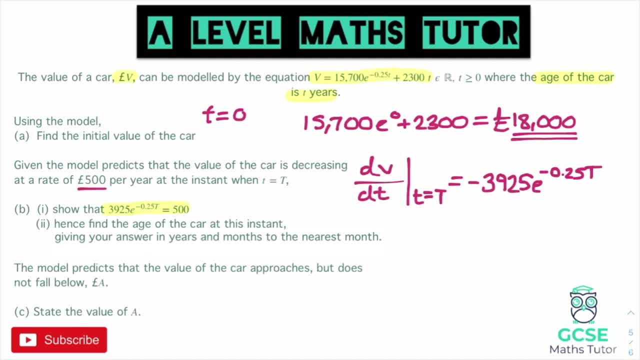 equal to the gradient that we've been told, and that is that it's going down by 500. so if we set that equal to 500, we would have negative 3925 e to the power of negative 0.25 t, and that is equal. 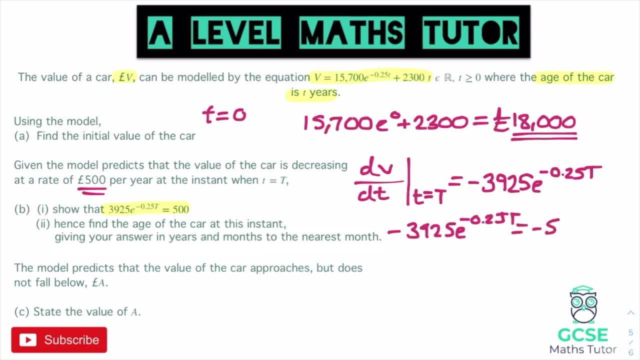 to negative 500.. Now we've got one step in order to make it look like how we've been asked to make it look like, and that is to divide both sides by negative 1. That would remove the negative from both sides, so our final answer would be positive. 3925 e to the power of. 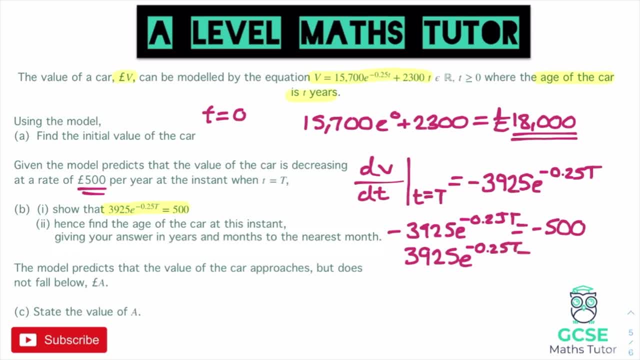 negative 0.25t and that is going to be equal to positive 500.. That is exactly what the question has asked us to show. so we have finished off our answer and we have shown what the question was asking for. Okay, so on to part two. It says here: hence find the age of the car at this instant. 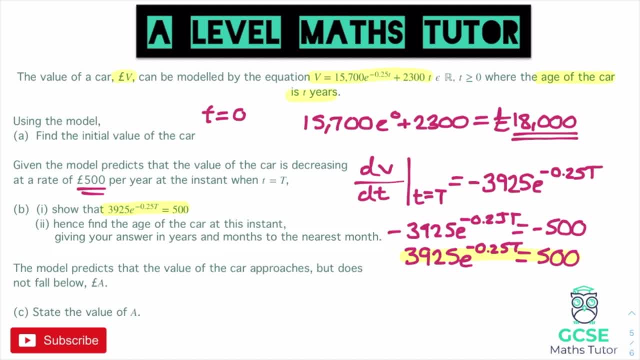 giving your answer in years and months to the nearest month. So for this particular part of the question, we have our equation to solve. We've just got that 3925e to the negative 0.25t is equal to 500. So we want to know the value of t at this instant. So the first thing that we can 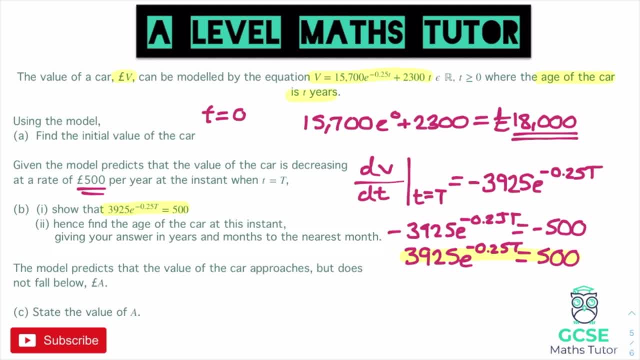 do, and if we carry on from our part one- and we'll just label this as part one, part i, and then we'll carry on here with part two- So the first thing that we're going to do is divide by the 3925.. 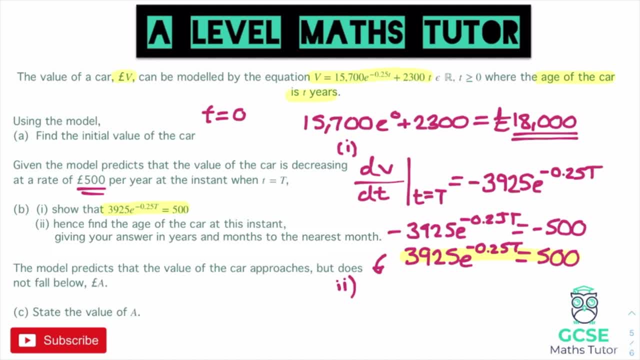 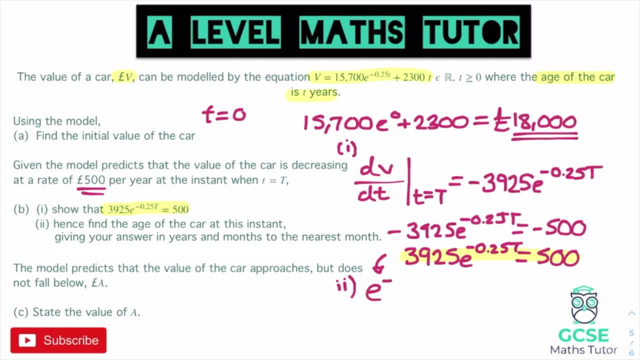 into our calculator e to the power of negative 0.25t And in fact we don't really need to type it in, because we could just write it as 500 over 3925.. So actually put the correct number there 3925.. So for the next step we want to remove the. 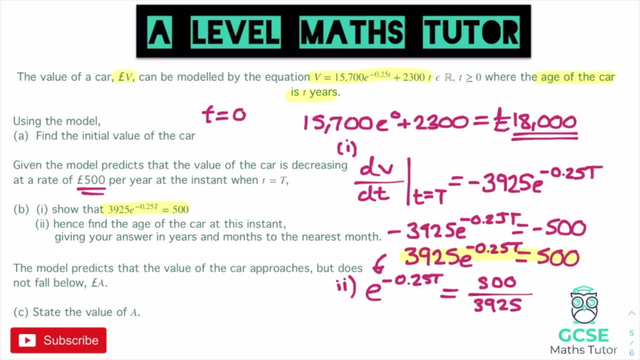 exponential. So if we take the natural log of both sides, we will have that negative 0.25t is equal to the natural log of- and we'll put this in brackets- 500 over 3925.. We now have one more step to get our value of t and that is to divide by negative 0.25. And if we do that, we'll write that. 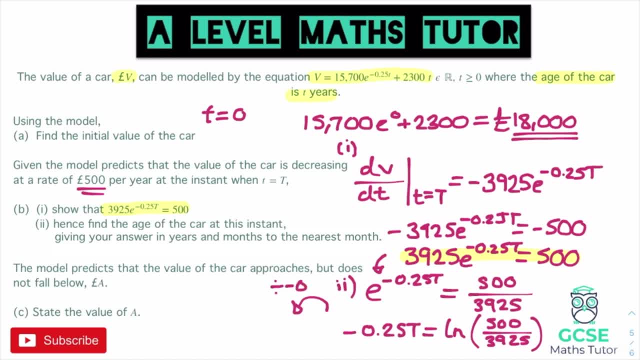 over here, divide by negative 0.25 and we get a value of t that is equal to. and what would it be? let's type it in our calculator, So the natural log of 500 over 3925, and then divide that by negative 0.25 and. 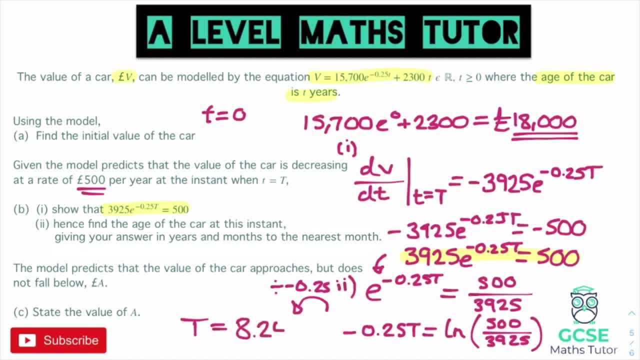 we get the answer 8.242.. A few more decimals here, so we'll leave it at 8.242.. And if we look at that there, that is in years, And remember it said that in the question and we highlighted that at the start, So that is eight and a quarter, or almost eight and a quarter years, and it does say: 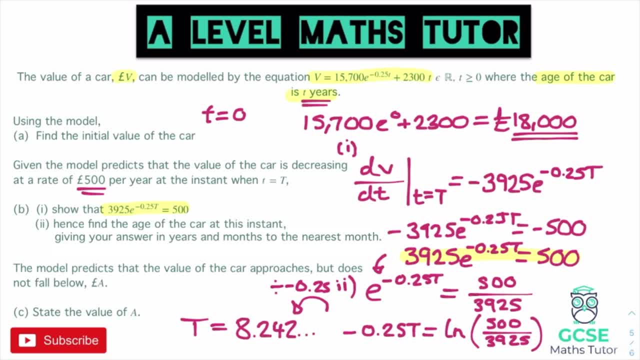 give it to the nearest month. So a quarter of a year would be equal to three months. So our answer for this here would be: eight years. There we go, three months, And that would be our final answer for part two of part b. So eight years, three months, and we'll just highlight that. 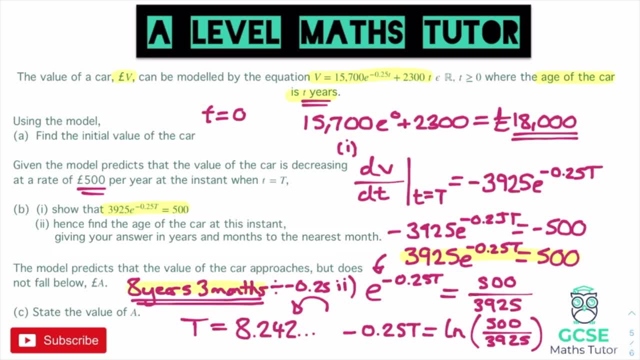 and that part is finished. Now for part c. it says the model predicts that the value of the car approaches but does not fall below a State, the value of a. Now, in order to do this, we need to think about what the exponential graph actually looks like. So if we do this and we can just about 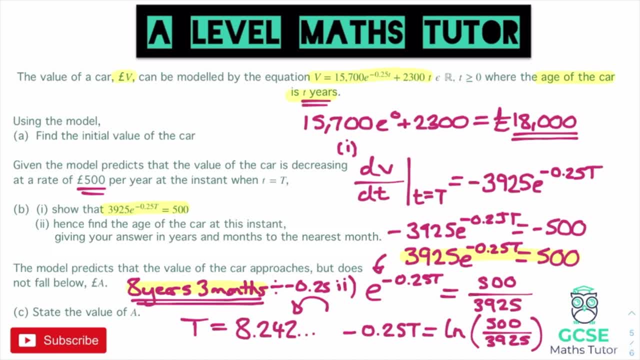 fit it in at the top here, if I get rid of. t equals zero. If we draw a small sketch of an exponential graph up here and we think about what it would look like, we know it is decreasing in value, So it would come down something like this: Now we would have an asymptote just up here, and if we 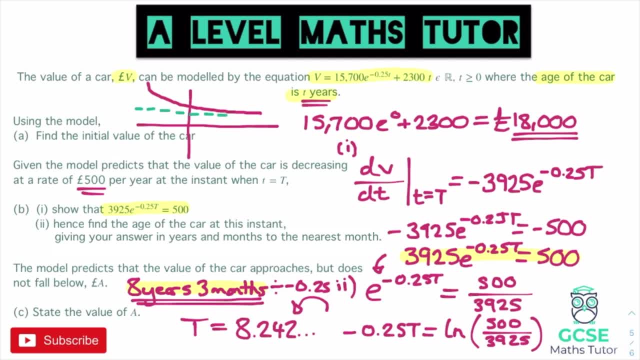 draw this in and think about the reason that I have drawn it up at the top there. The reason I have drawn it up at the top is because our exponential has this plus two thousand three hundred, just at the end. Now that means it has been translated upwards and this value here would 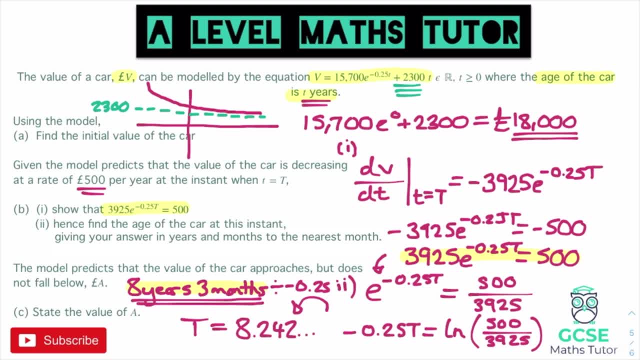 be two thousand three hundred. So, as it has moved up from here, we have a value of two thousand three hundred. That means it is never going to approach. Well, it's going to approach, but it is never going to fall below two thousand three hundred. So the value of a to finish this question would be two. 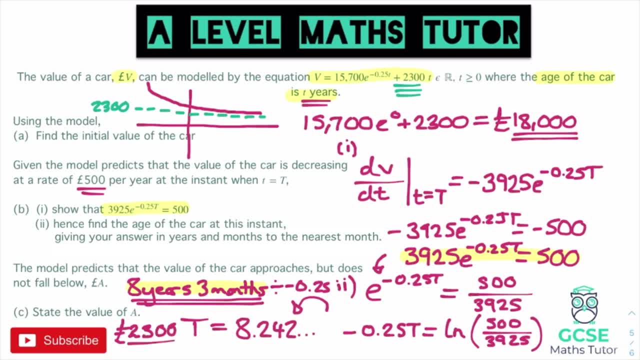 thousand three hundred pounds. We'll write this down the bottom, We'll highlight that as our final answer and there we go, And that is looking at modelling with exponentials. Okay, so that is the end of the video, looking at exponentials. Obviously, if you haven't already, go and check out the video. 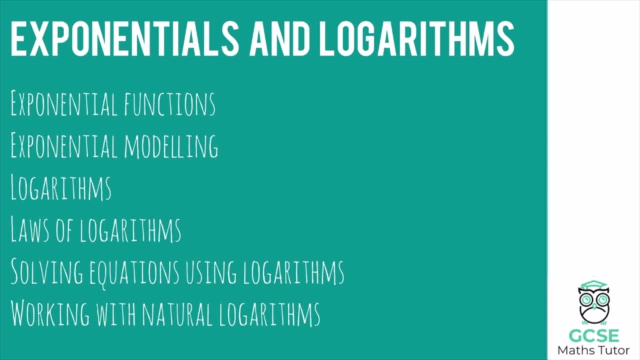 on logarithms or check out our other videos on logarithms. So if you haven't already, go and check out any of the other videos in the description. looking at the other chapters, This is obviously the final chapter on the AS Pure Maths curriculum, So do make sure that you follow along with any of 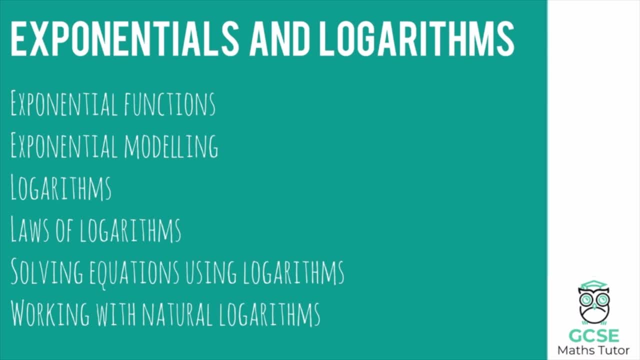 the other videos and be in tune for obviously, some of the other videos I'm going to have coming out looking at some of these topics in a little bit more depth, But that is obviously the last one, so please do like the video, Please subscribe, Please leave me a comment if you have enjoyed any of this. 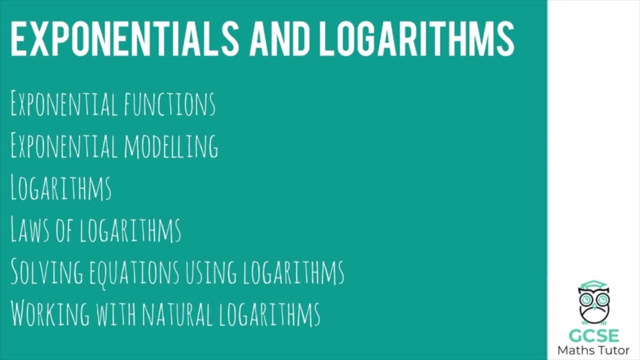 series and let me know anything that you'd be looking for next. But until the next one, I will see you for the next topic. Thank you for watching and I will see you in the next video.